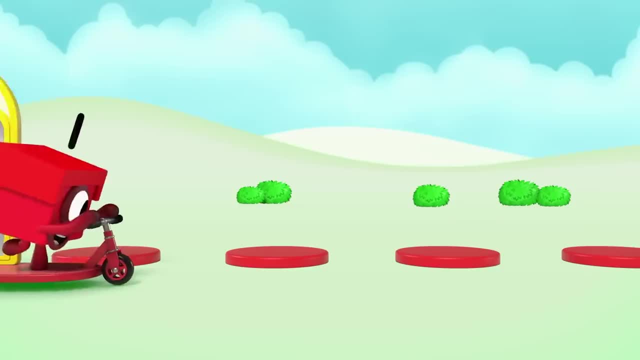 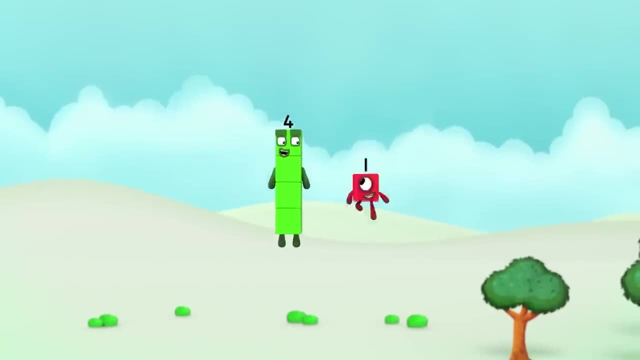 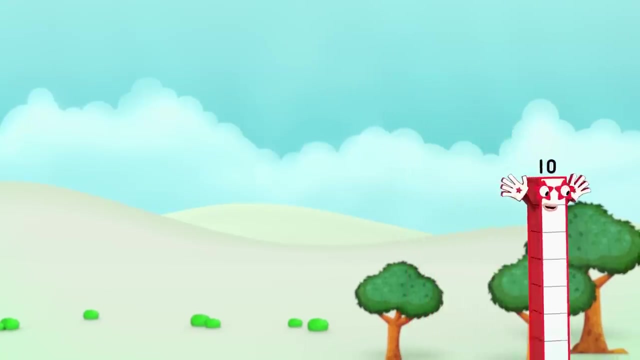 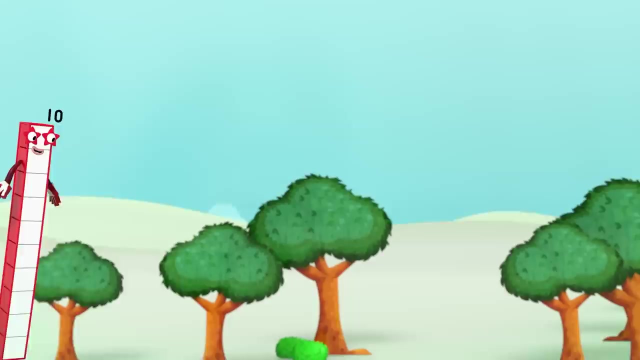 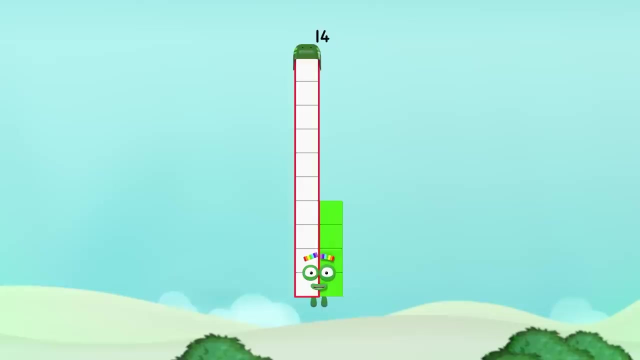 Zero One, two, three, four, five, six, seven, eight, nine, ten Coming in for landing. Keep going, Every second counts And clear for launch. Eleven, twelve, thirteen, Fourteen, Fourteen. 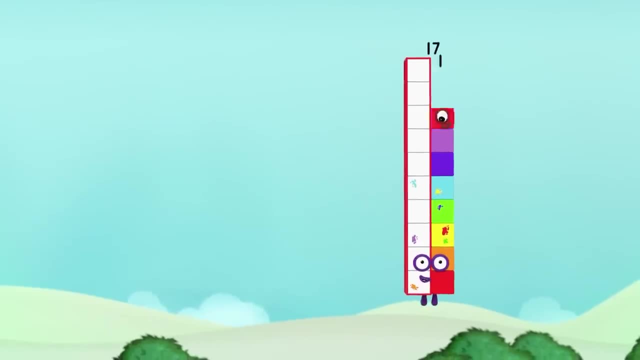 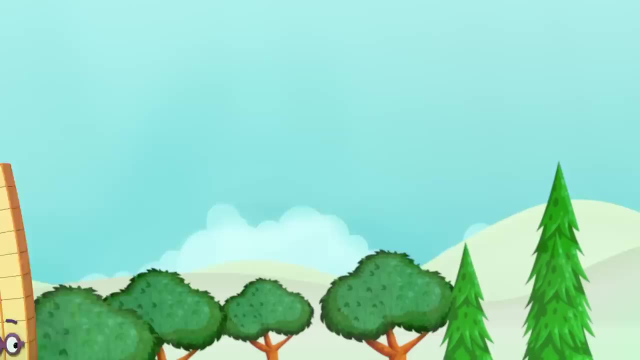 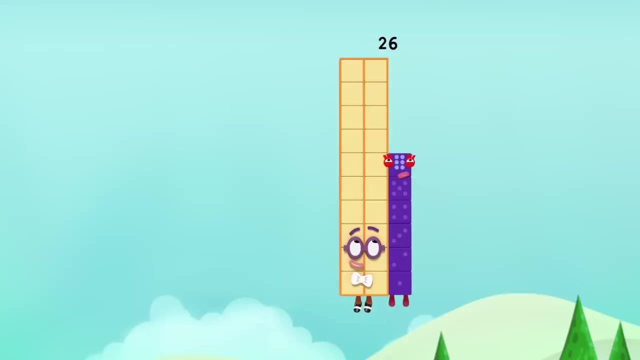 Fifteen, Sixteen, Seventeen, Eighteen, Nineteen, Twenty- We're going to make so many new friends today. Whee, Twenty-one, Twenty-two, Twenty-three, Twenty-four, Twenty-five, Twenty-six, Twenty-seven. 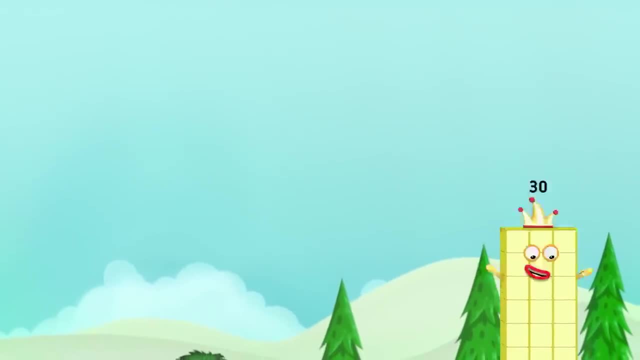 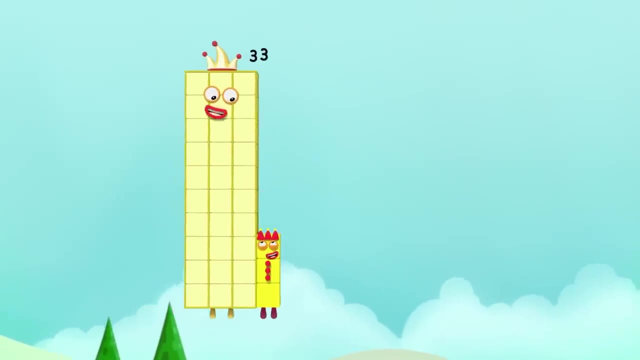 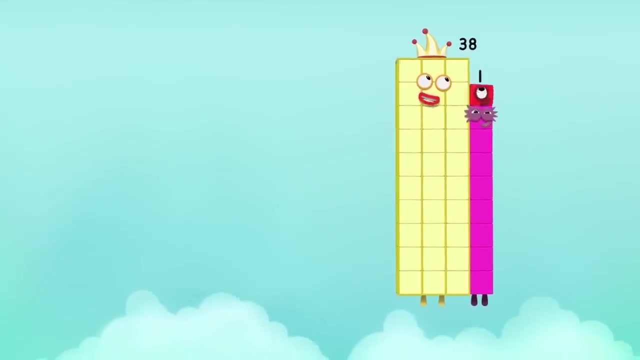 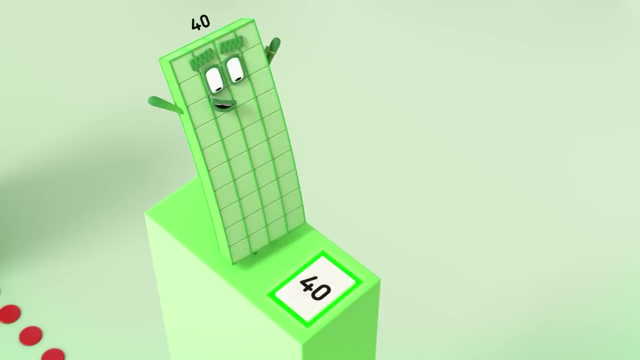 Twenty-eight, Twenty-nine, Thirty, Excellent acrobatics. everybody On with the show. Thirty-one, Thirty-two, Thirty-three, Thirty-four, Thirty-five, Thirty-six, Thirty-seven, Thirty-eight, Thirty-nine, Forty, Ooh, I like the flipper. It's rectangular. 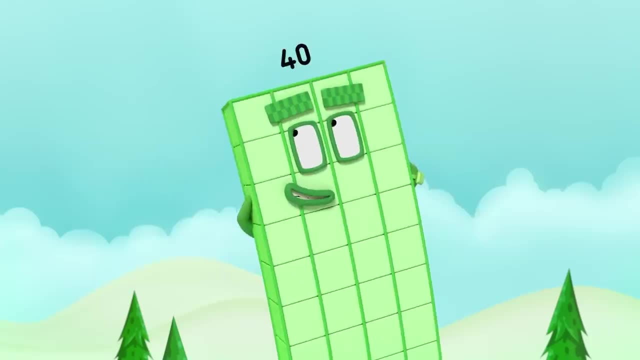 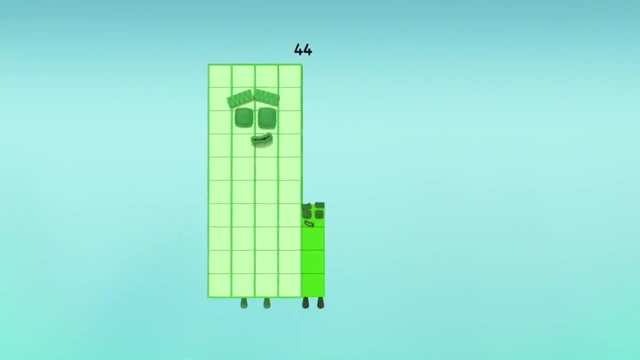 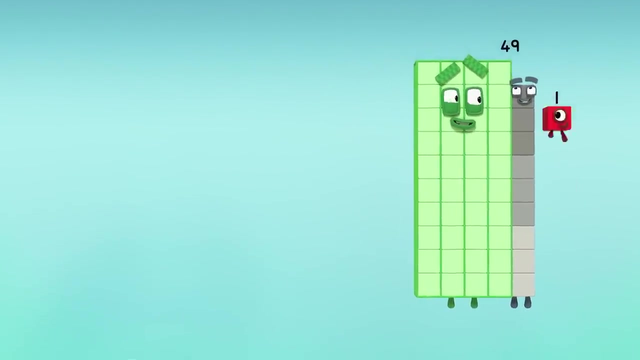 Stay focused. We can do this, Sorry. Forty-one, Forty-two, Forty-three, Forty-four, Forty-five, Forty-six, Forty-seven, Forty-eight, Forty-nine, Forty-eight, Forty-nine, Forty-nine, Fifty-one, Fifty-two. 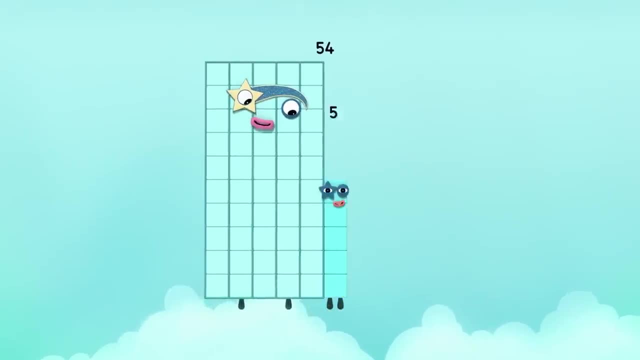 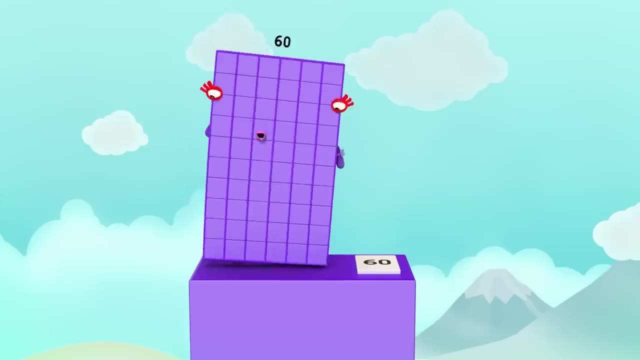 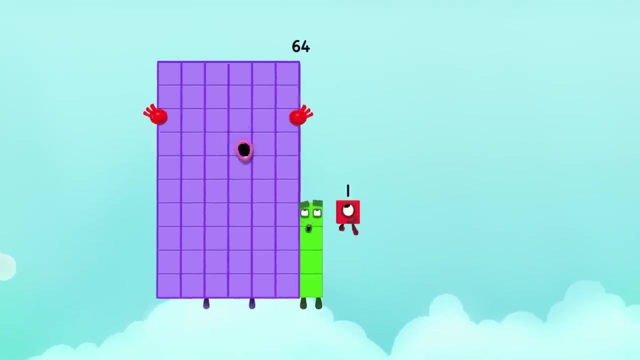 Fifty-three, Fifty-four, Fifty-five, Fifty-six, Fifty-seven, Fifty-eight, Fifty-nine, Sixty. Racing through the sky, this high roller's gonna fly. Sixty-one, Sixty-two, Sixty-three, Sixty-four. 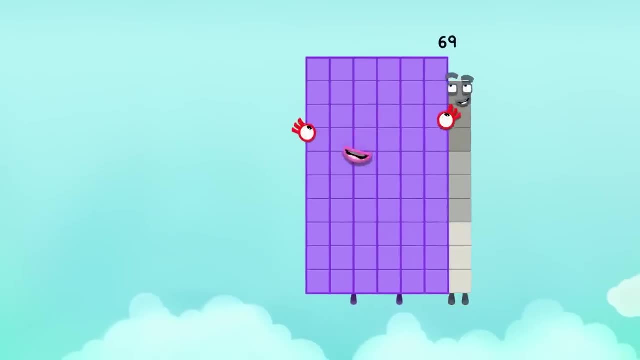 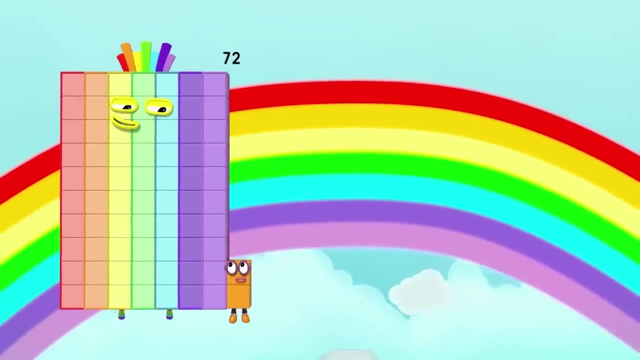 Sixty-five, Sixty-six, Sixty-seven, Sixty-eight, Seventy. We're going over the rainbow. Seventy-one, Seventy-two, Seventy-three, Seventy-four, Seventy-five, Seventy-six, Seventy-seven. 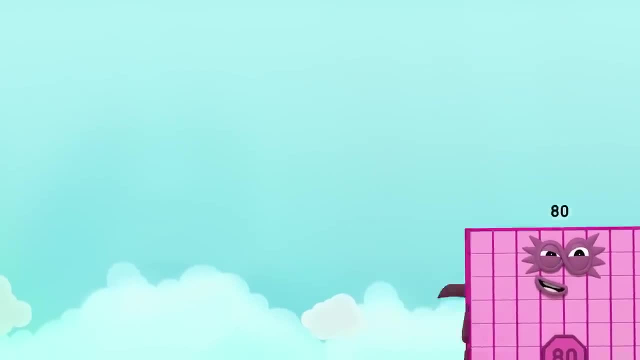 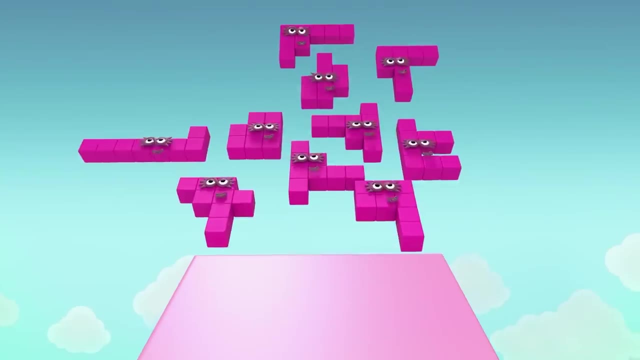 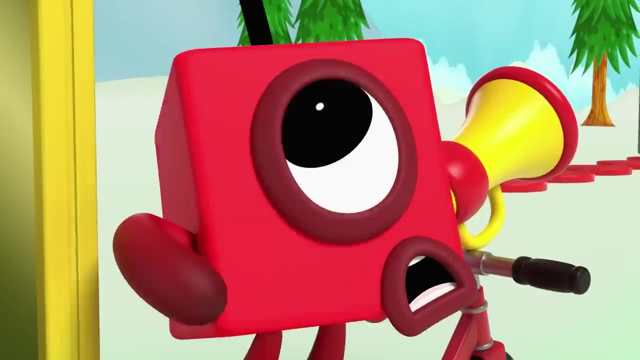 Seventy-eight, Seventy-nine, Eighty. I don't like the look of those clouds. There's no time to stop Octoblocks, assemble Dinoctoblock roar, Roar Up up and away. 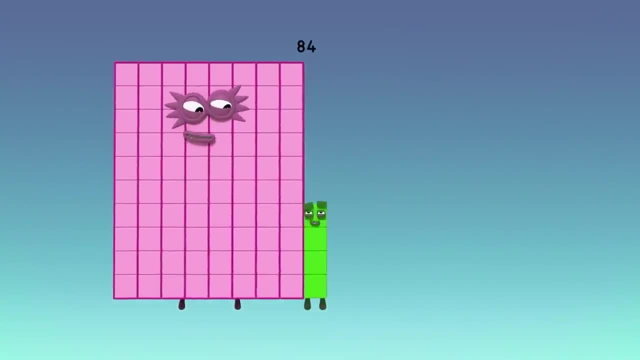 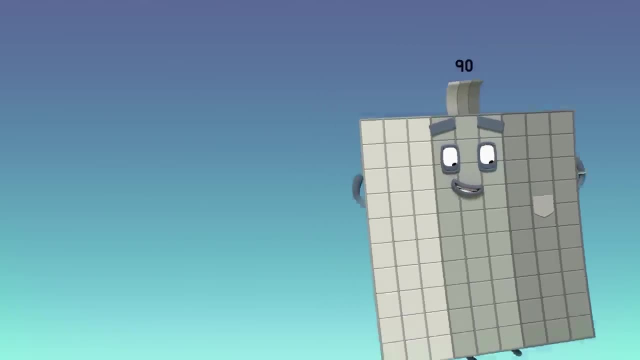 Eighty-one, Eighty-two, Eighty-three, Eighty-four, Eighty-five, Eighty-six, Eighty-seven, Eighty-nine, Eighty-nine, Ninety. Nearly there, with no time to spare, This should do the trick. 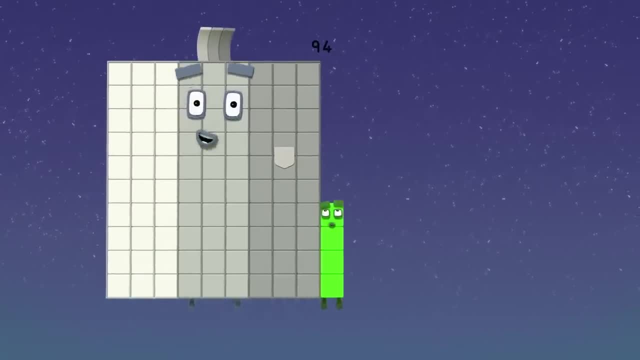 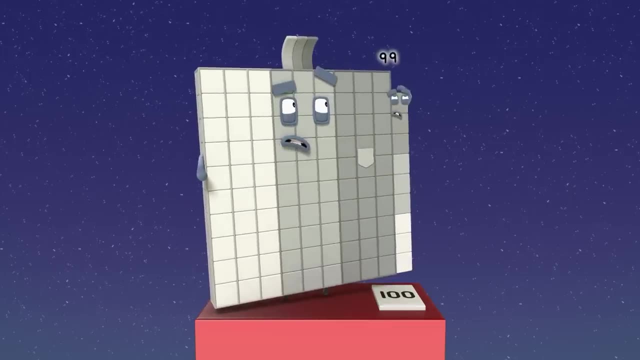 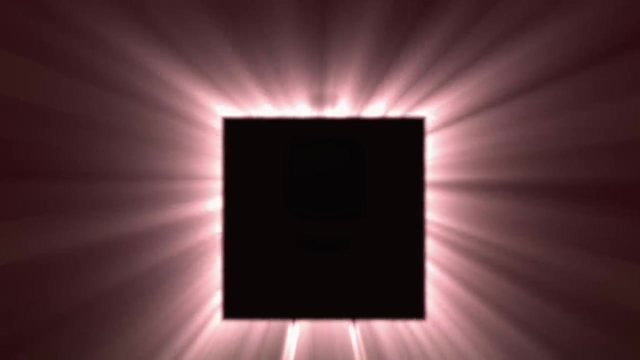 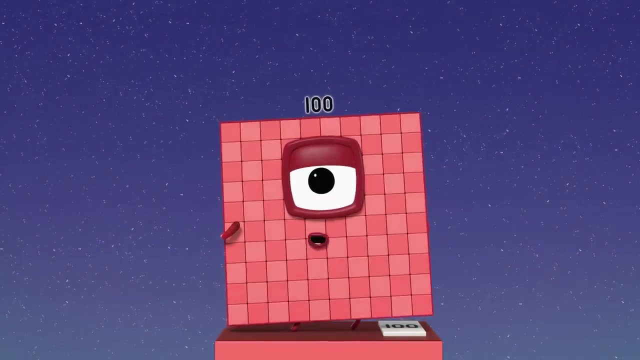 Ninety-one, Ninety-two, Ninety-three, Ninety-four, Ninety-five, Ninety-six, Ninety-seven, Ninety-eight, Ninety-nine And one more is Roar One hundred, I am one hundred. 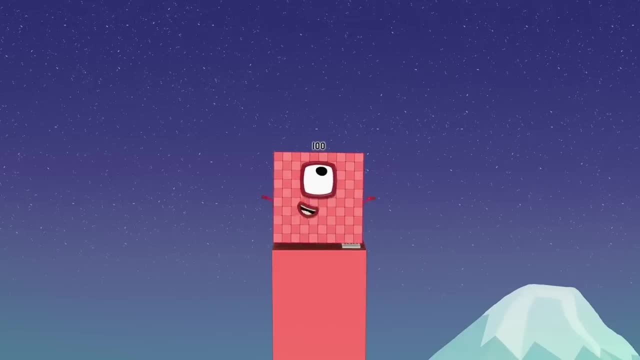 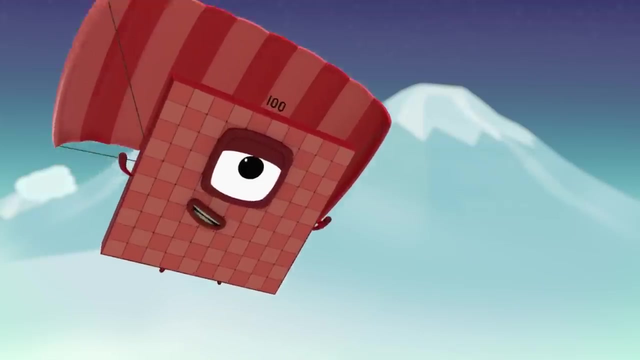 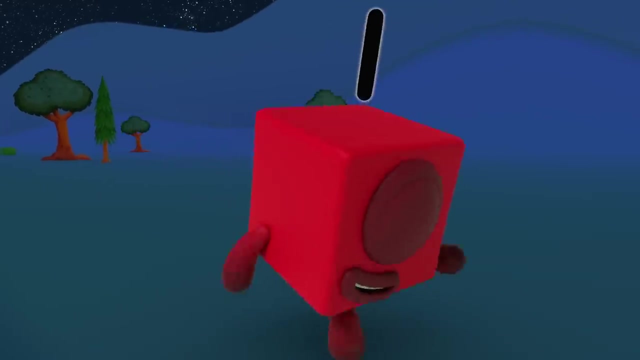 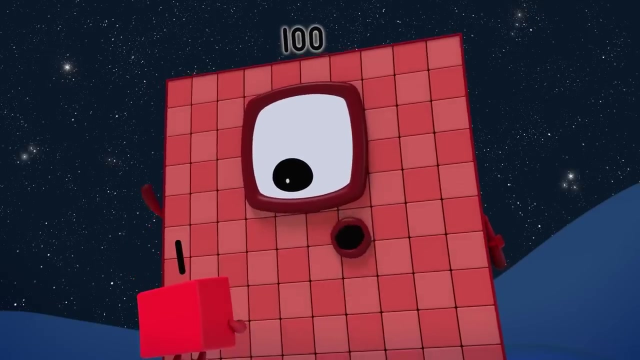 Ten, lots of ten on top of the world. Now, how do I get down again? Ah, a parachute. One hundred is A parachute once. Hooray, Hooray, One hundred is here. One, One hundred, Hello one. 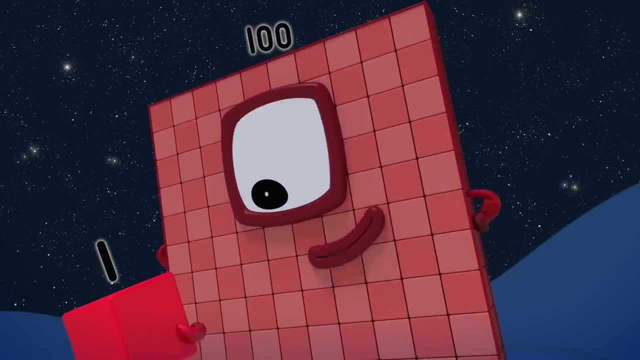 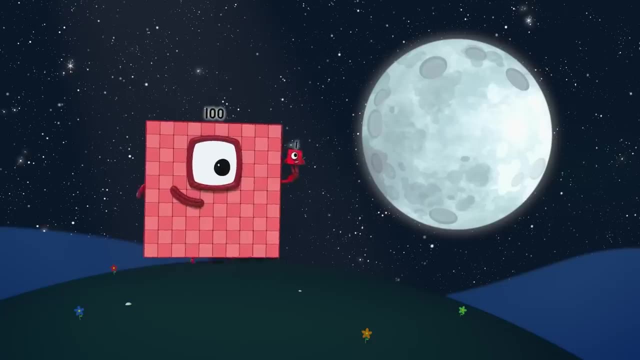 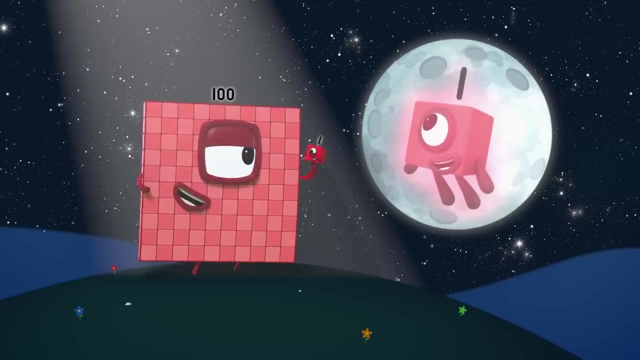 You're so big. Yes, little one, I'm a big number, But I wouldn't be here at all if it weren't for you. Look how far we've come. Remember when there was only one, Then ten ones made one ten. 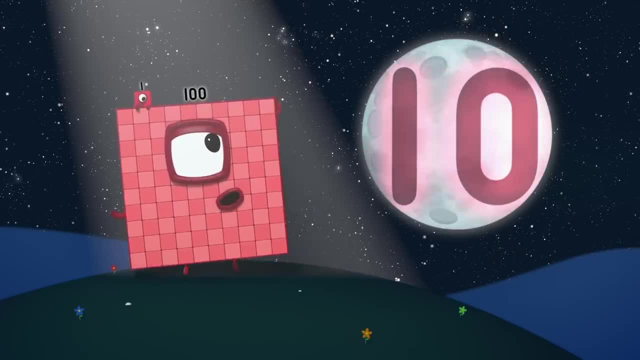 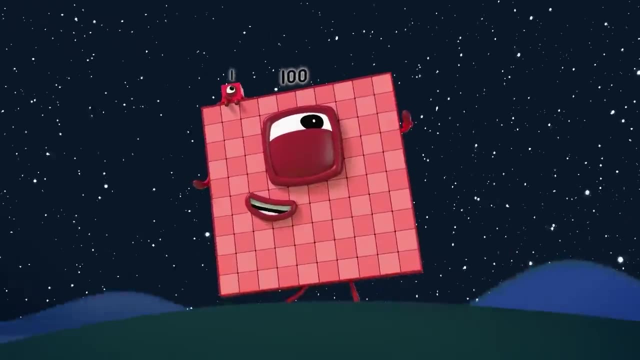 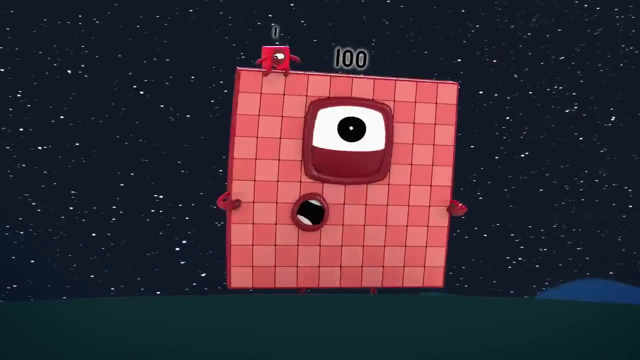 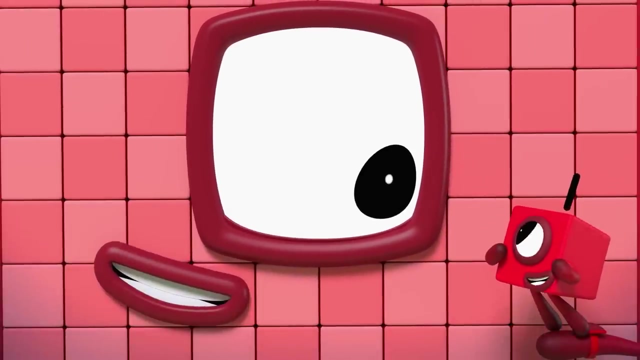 With a one and a zero. Now we've reached a new place, A place of possibilities, A new friend, a new face And a brand new kind of hero. I'm big, So big. I'm really, really, really big. 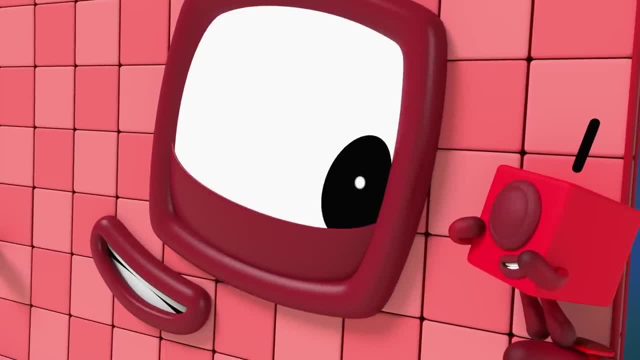 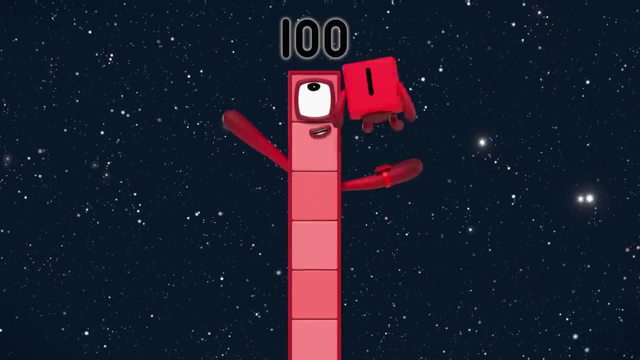 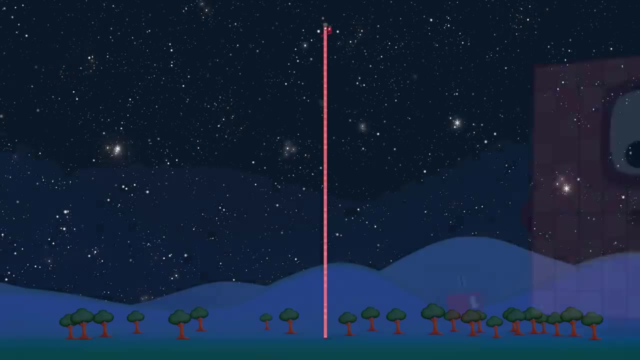 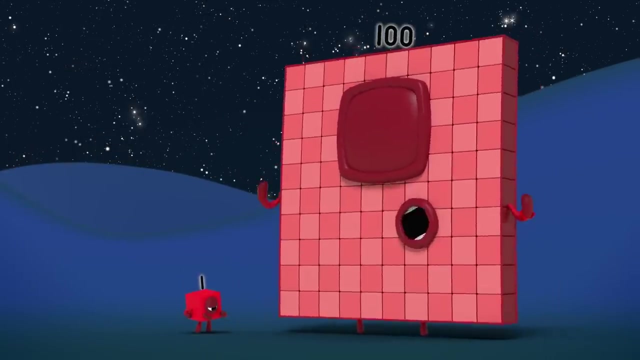 I'm gigantic Gigantic. Did I mention I was big? I'm taller than the tallest tree. No one here's as tall as me Because I'm big. I'm really very big. One, two, three, four, I'm so big. you'll need a quicker way to count. 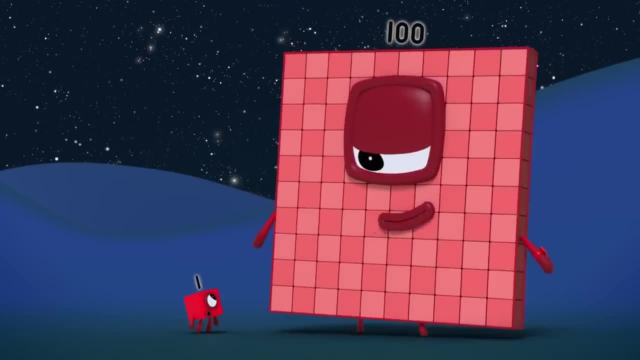 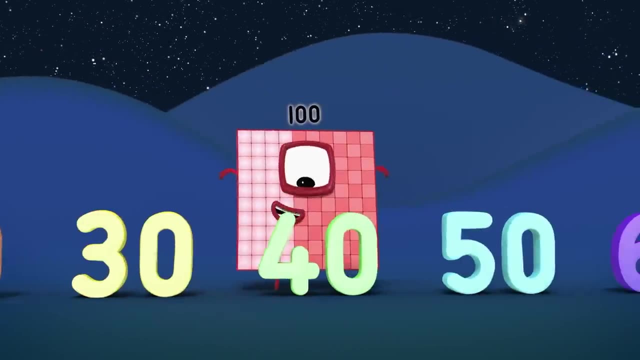 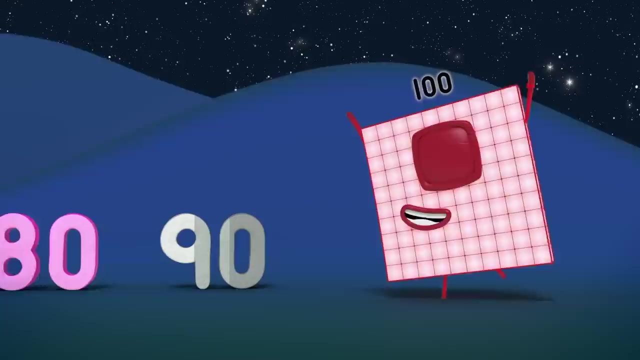 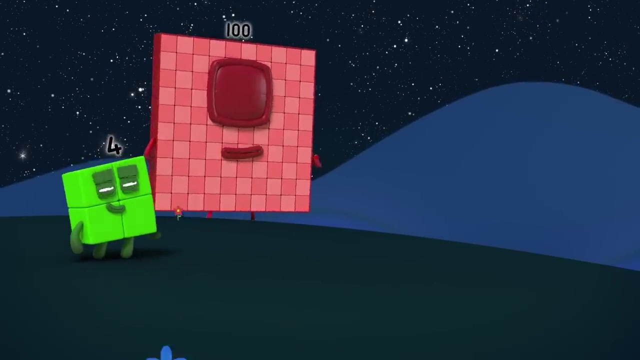 If you count ten, tens, one, ten at a time, You'll reach the right amount: Ten, twenty, thirty, forty, fifty, Sixty, seventy, eighty, ninety, One hundred. She's square. I'm ten by ten. 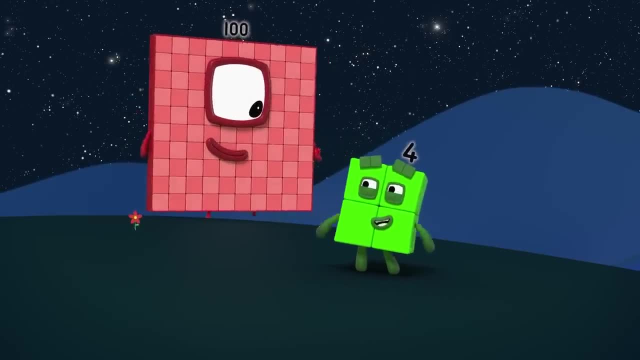 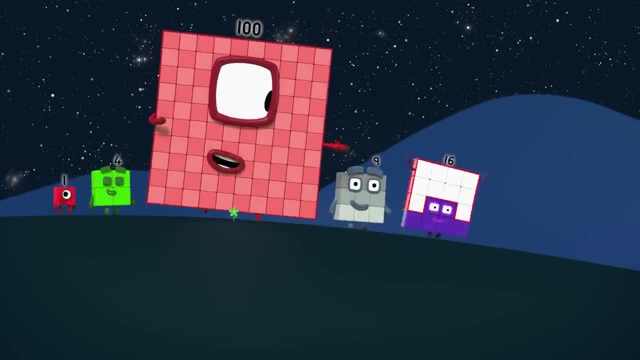 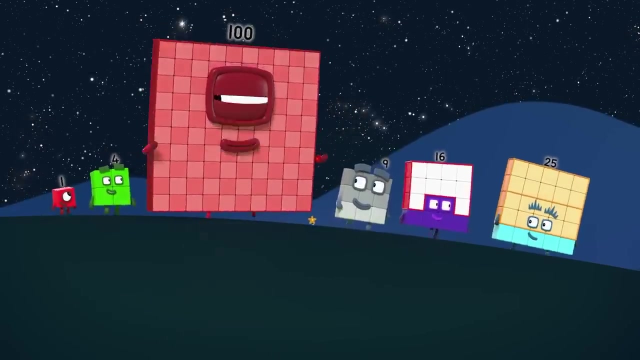 That makes me square. She's impressive. Now I've noticed that she's square One, four, nine, sixteen, twenty-five. You'll know when all the squares arrive, Because I'm square, I'm one big, massive square. She's square. 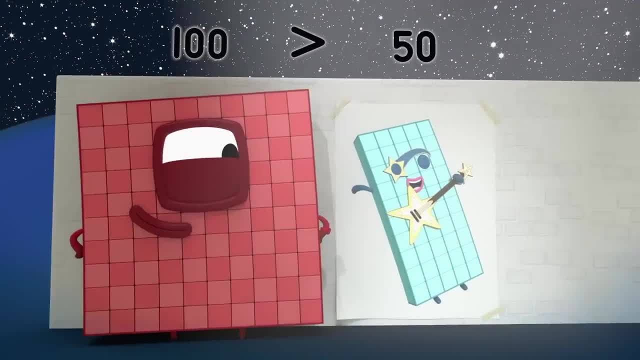 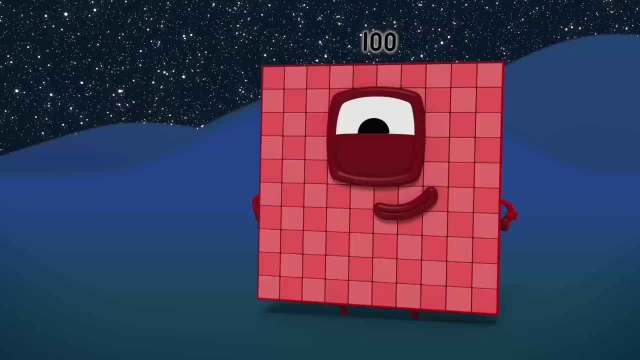 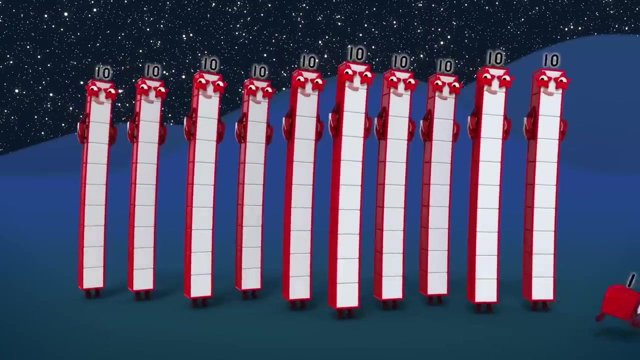 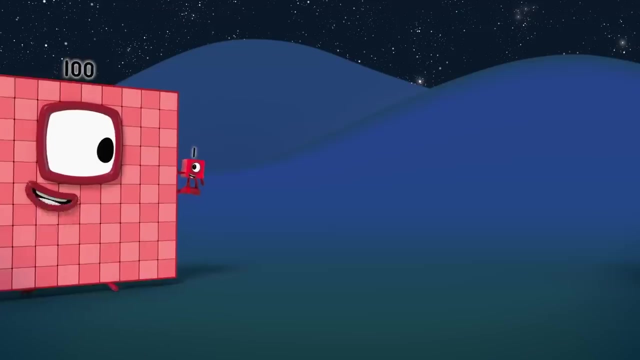 You can't help being quite impressed. She's the greatest. She's greater than the rest. She's ten times ten, as you can see, A hundred times the size of me. She's great. We all think she's the best, But I'm still one of you. 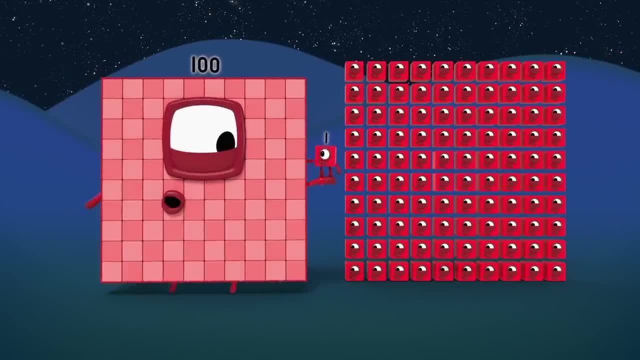 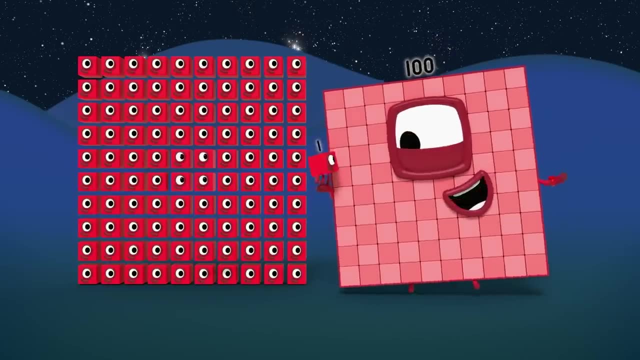 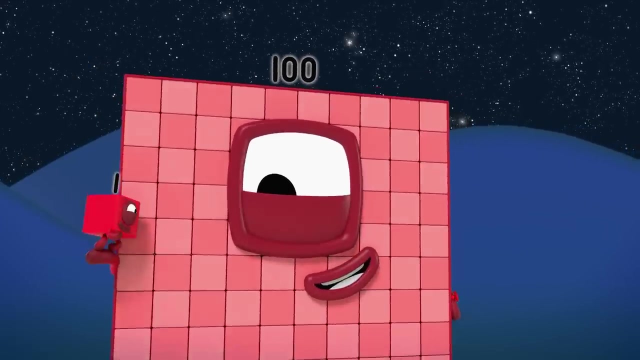 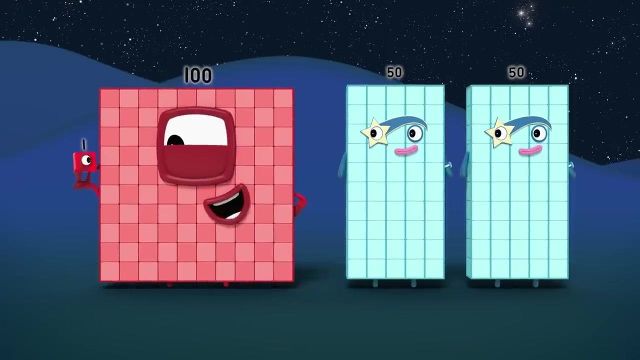 I'm one with you. It takes a hundred ones to make one me. I won't make fun of you. I'm not done with you Inside. I'm just like anyone you'll see. But I'm big. I'm really really somewhat big. 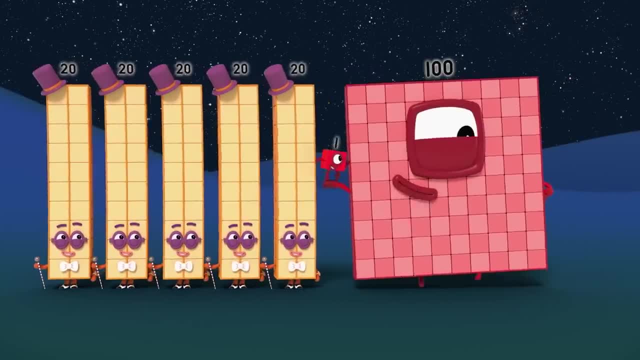 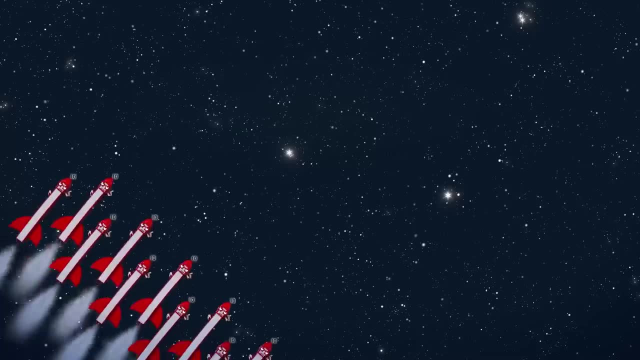 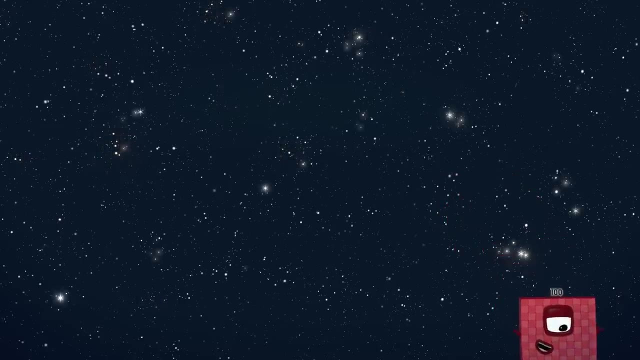 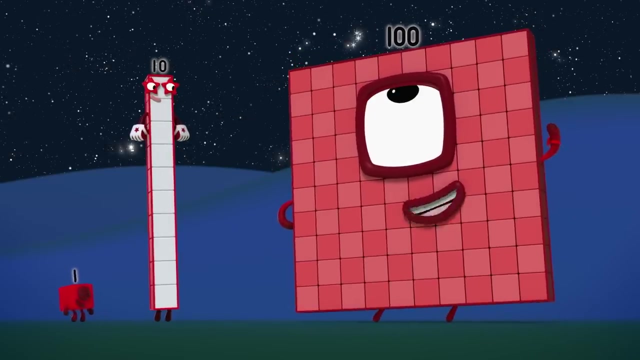 I'm tremendous, She's tremendous. I'm proud that I'm so big. You'll see ten tens as we fly by, Ten rockets shooting through the sky. That's big, Unquestionably big. I'm bigger Because I've got three figures. 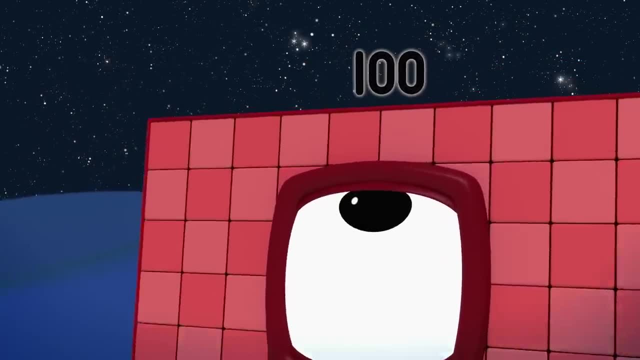 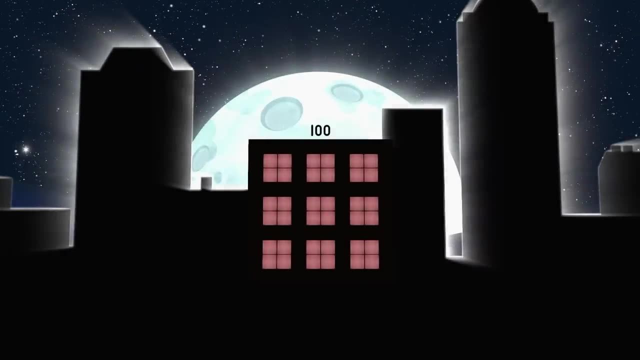 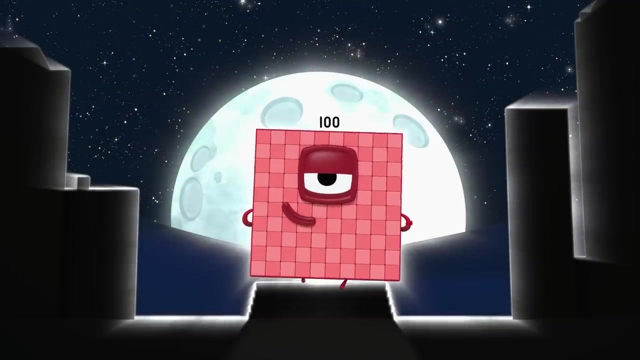 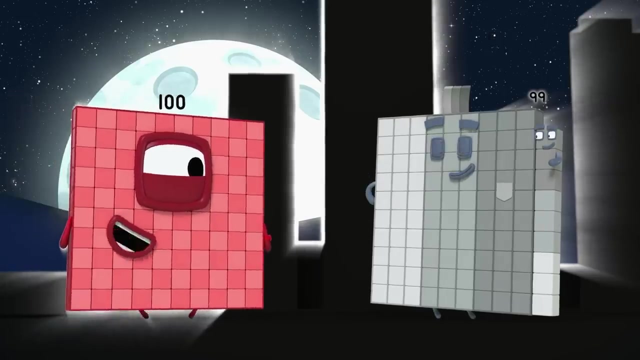 My zeros might give you a clue. Is this the start of something new? I'm big. I'm really really, really big. I'm a landmark. You can't miss me. I'm that big And life's a hundred times more fun. 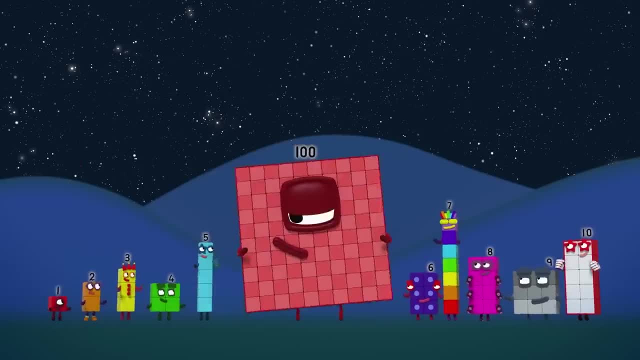 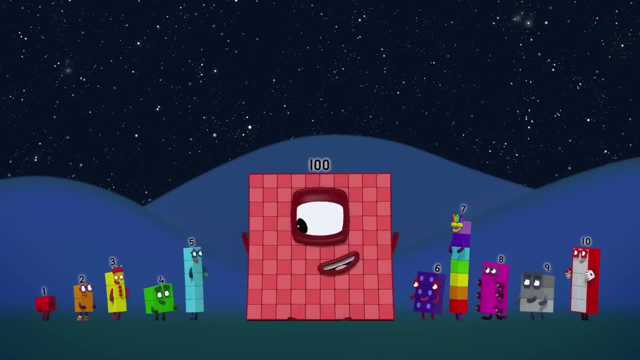 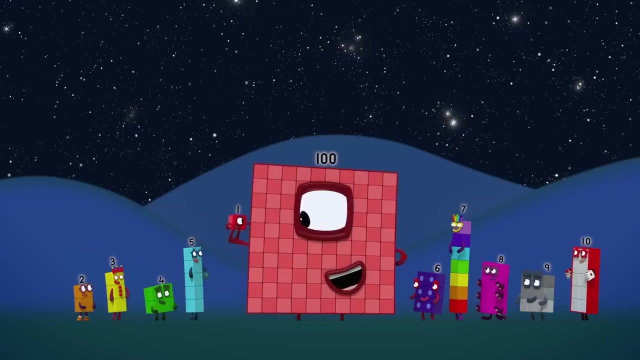 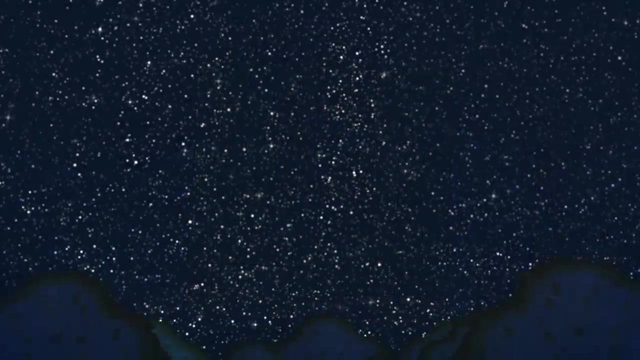 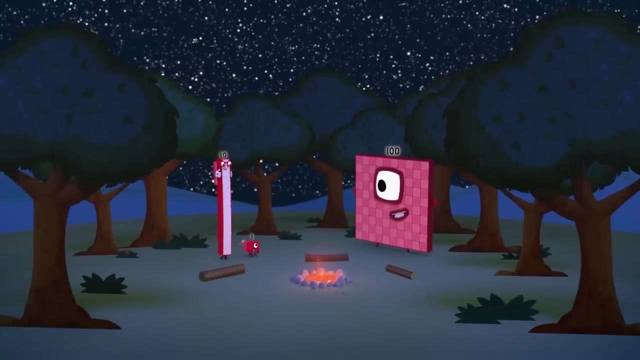 When you're ninety-nine plus one. I'm big, She's tremendous. I'm big, She's tremendous, I'm really, really, really very big. Hello one, Hello ten, Hello one hundred Sit. sit. 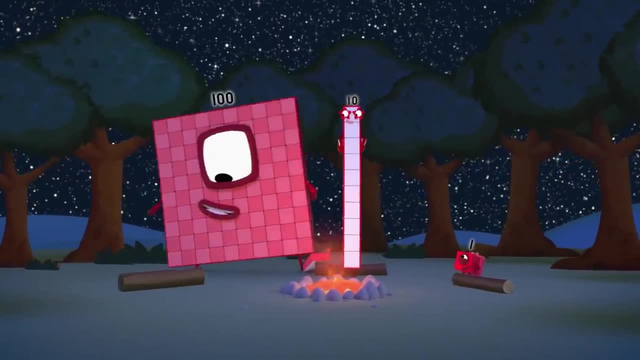 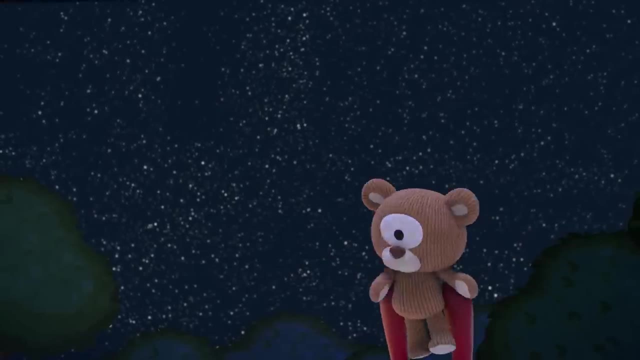 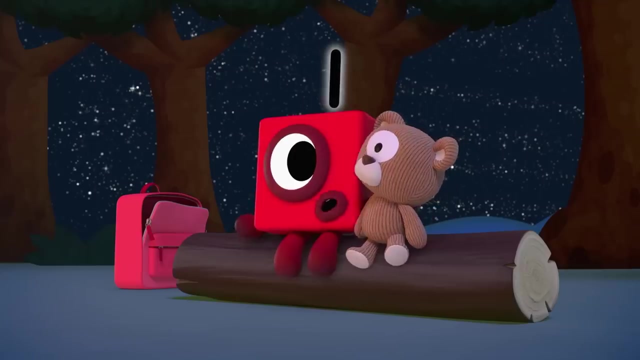 One's place, ten's place, hundred's place. Look, Teddy, so many stars. There must be a hundred of them. Oh, there are many more than that, More than one hundred, But you're the biggest number I know. 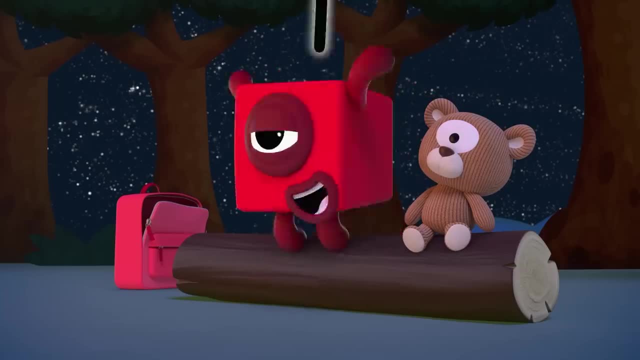 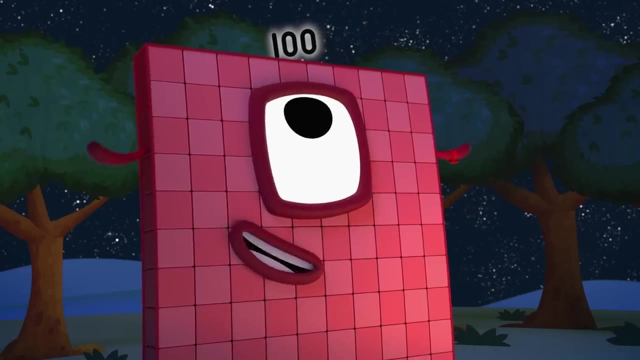 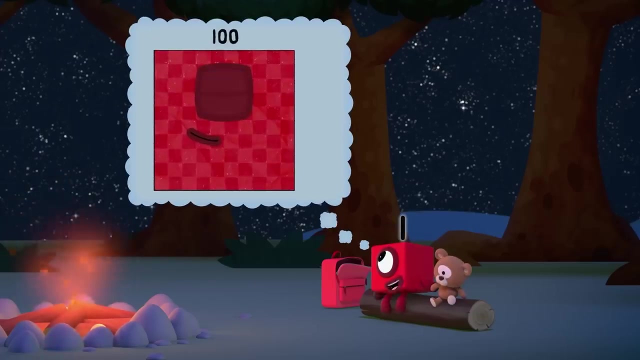 You can always make a bigger number by adding one. And how would that look? Think, think big. This is a good night for big thoughts. Oh, I love thinking about numbers. Look one hundred. if I join up with you, we'll be. 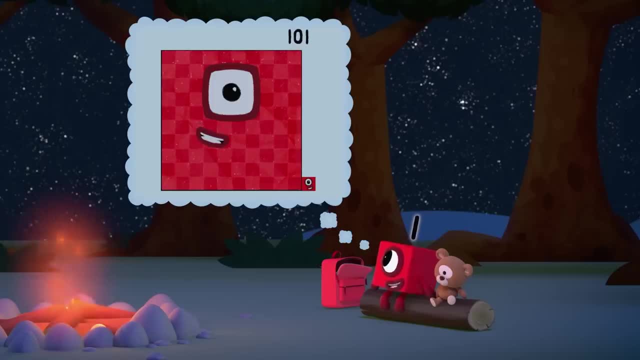 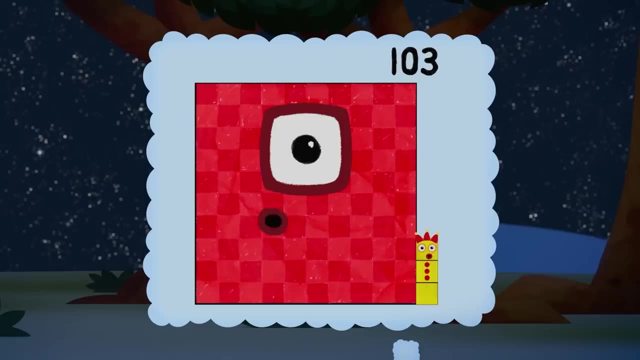 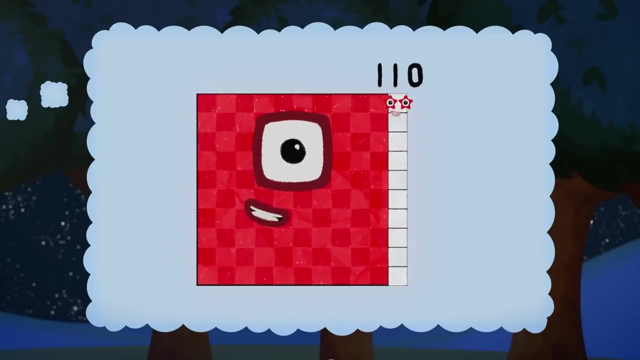 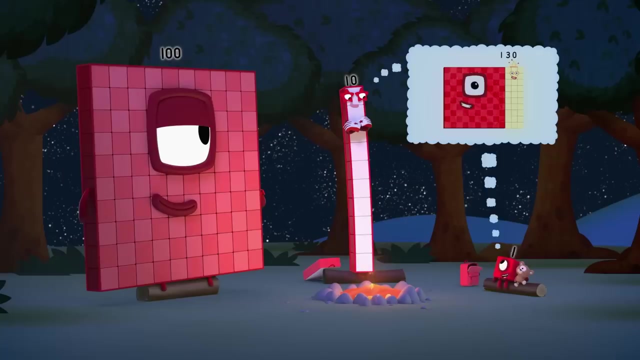 One hundred and one, And we can keep adding one, One hundred and two, One hundred and three, Or we can add tens, One hundred and ten, one hundred and twenty one hundred and thirty. And if we can add ones and tens, we can add hundreds. 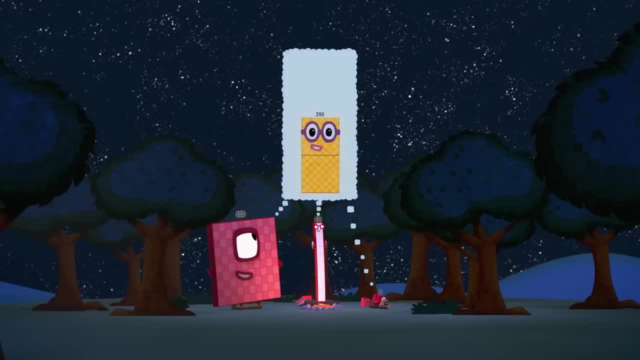 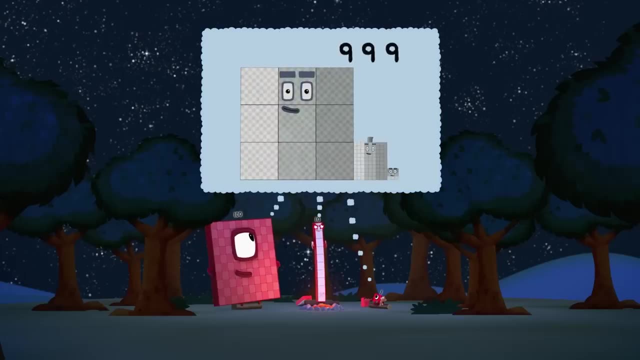 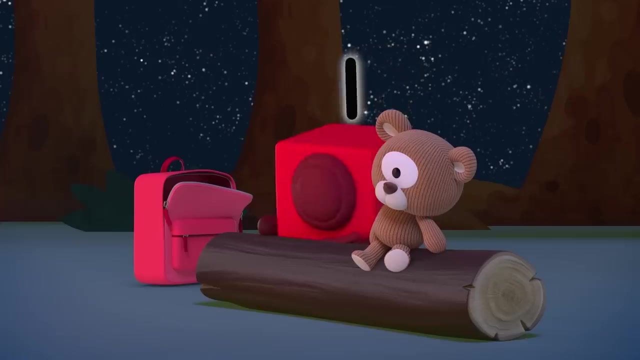 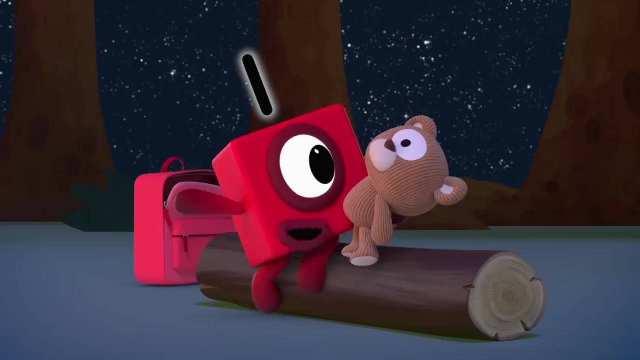 One hundred two hundred three hundred, We could make Nine hundred and ninety-nine. Nine, Wow, that's the biggest number I can think of, But there must be bigger numbers because we can always add more blocks. So what's bigger than nine hundred and ninety-nine? 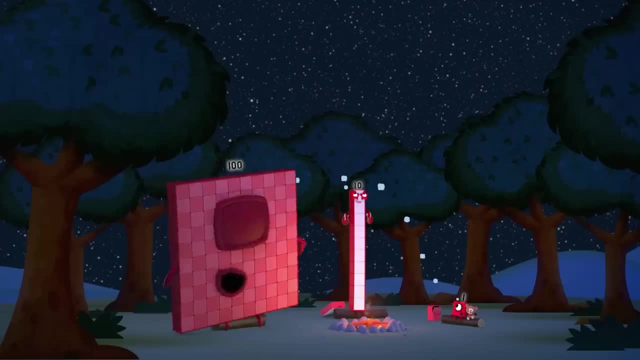 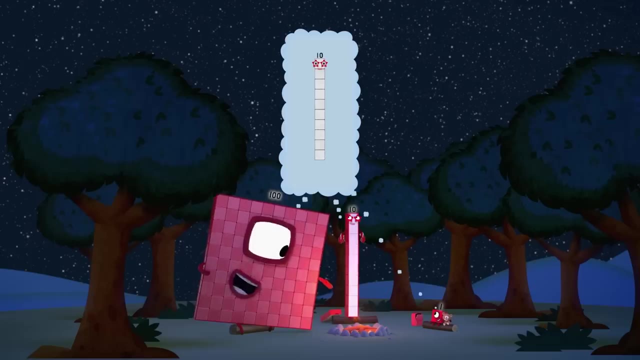 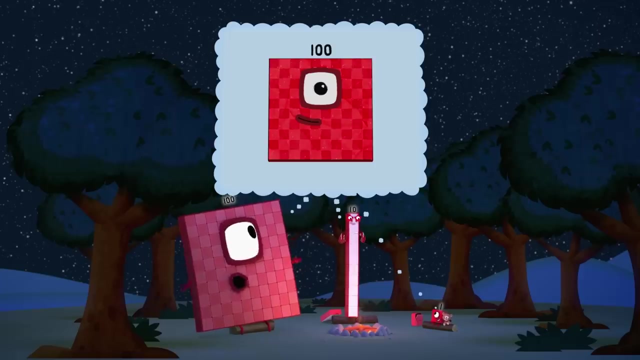 Think about it this way: Let's start with you. One One block, Now ten of you, Ten ones. What's that? Ten? Now let's have ten tens, What's that? One hundred, Now Ten hundreds, What's that? 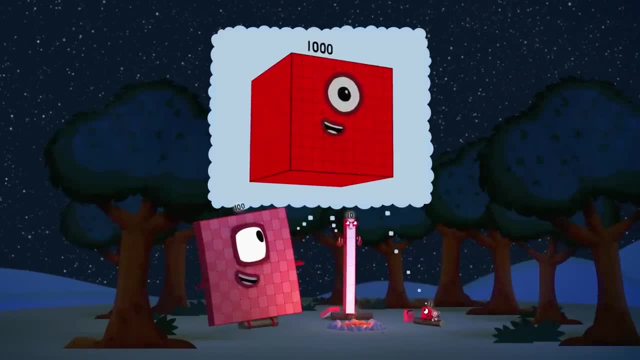 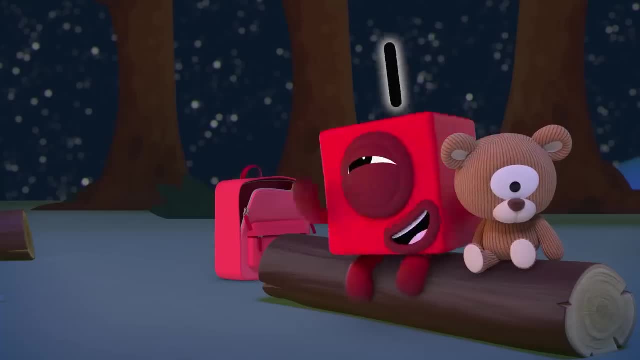 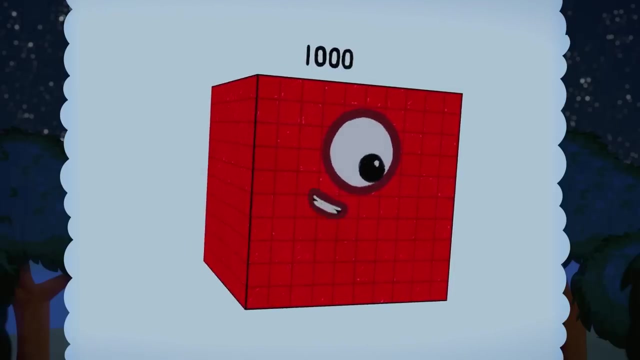 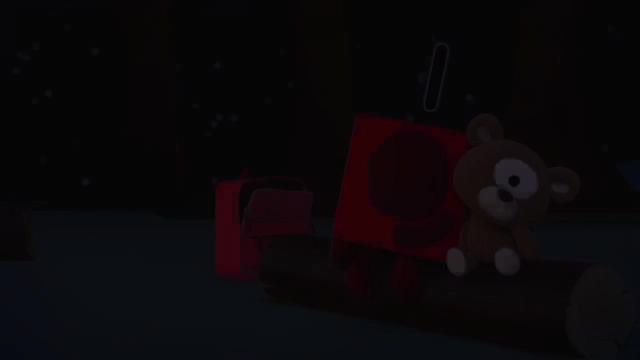 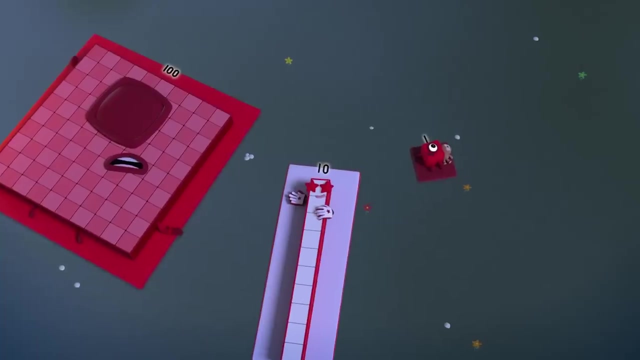 One thousand. You look like a giant, me. I'm a thousand ones. Wow, I can't wait to meet you. Oh, Good night, little one. Good night one thousand. There are so many big thoughts buzzing in my head I'll never get to sleep. 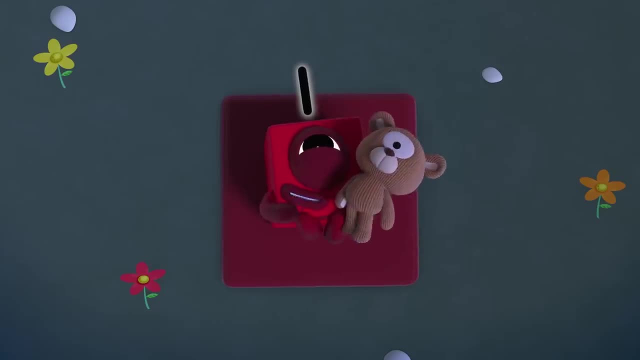 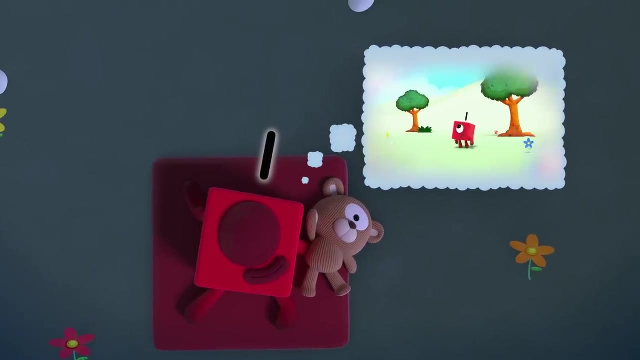 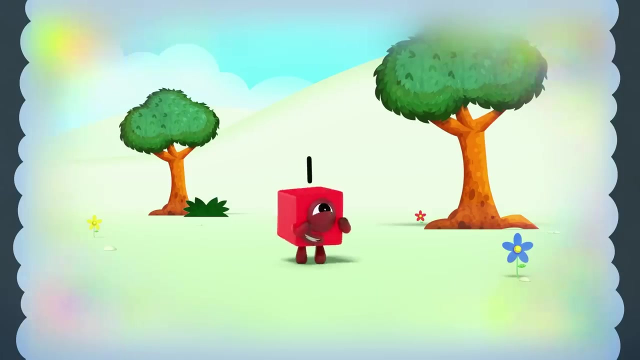 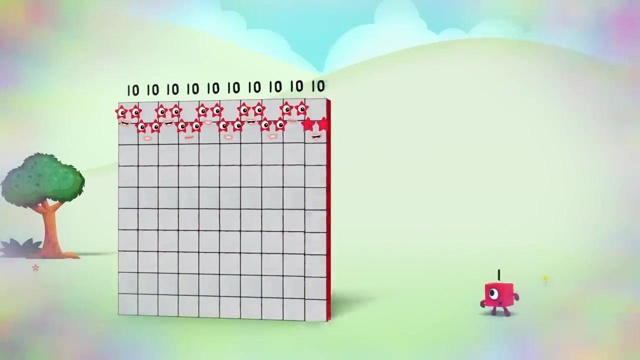 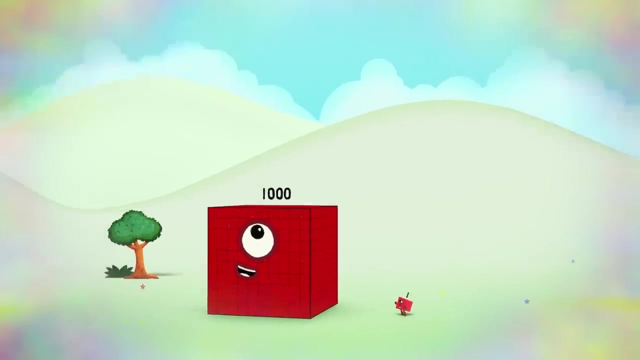 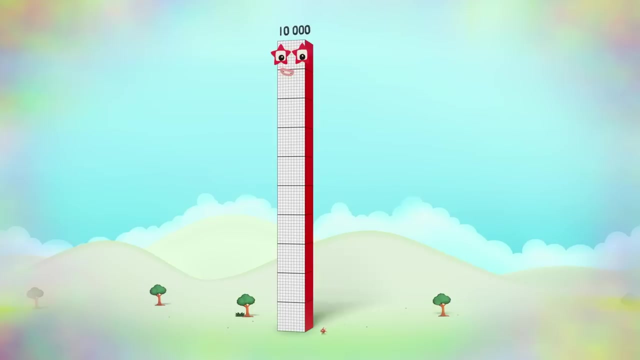 Ten hundreds are one thousand, And that's not even the biggest number. Oh One One dream, Hello dream. Ten ones are ten, Ten, tens are one hundred. Ten hundreds are one thousand. Ten, lots of one thousand are Ten thousand. 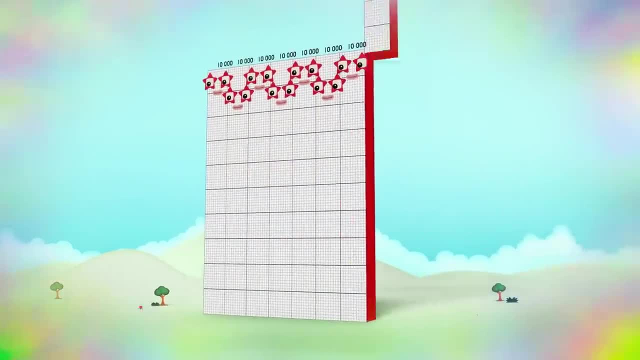 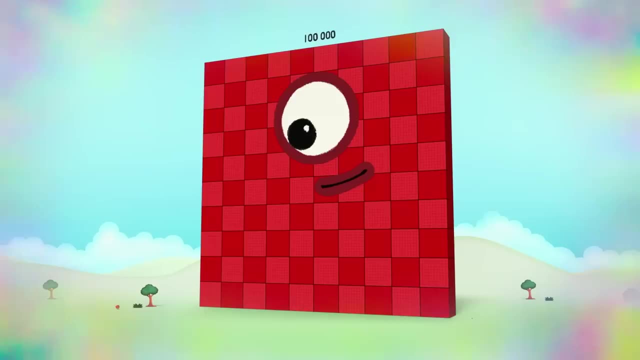 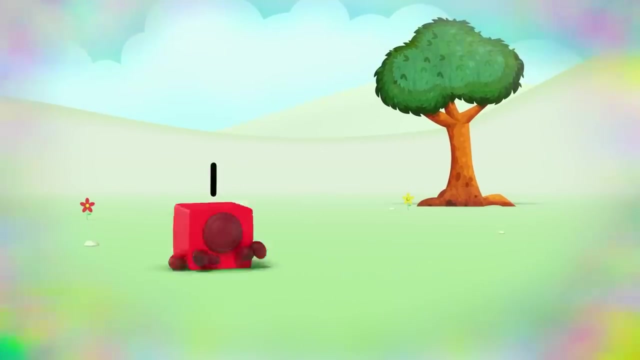 Ten lots of ten thousand, And ten lots of one hundred thousand are One hundred thousand, And ten lots of one hundred thousand are One million. Hello, Hello, little one. Wow, I never knew there was a number so big, And you can always make a number that's bigger. 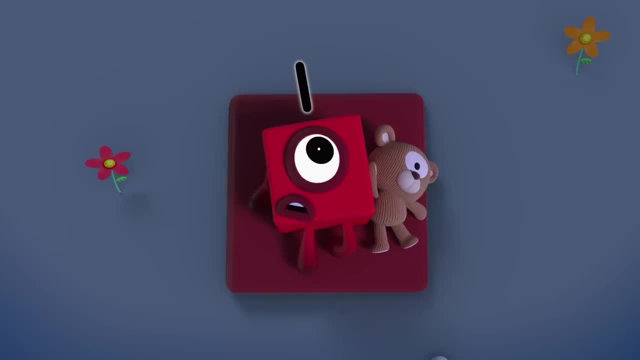 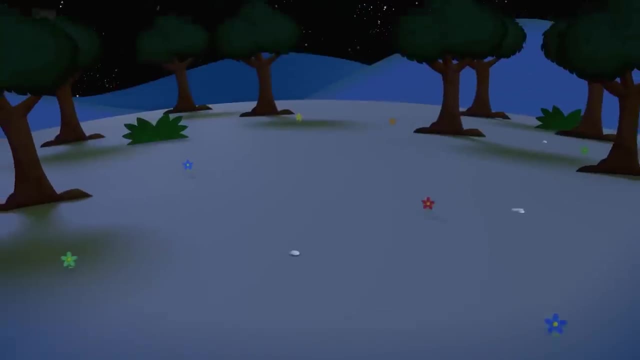 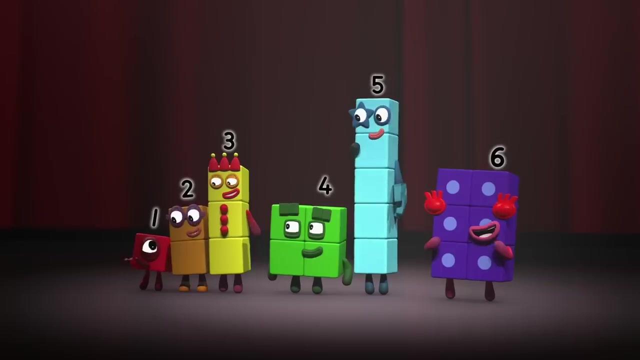 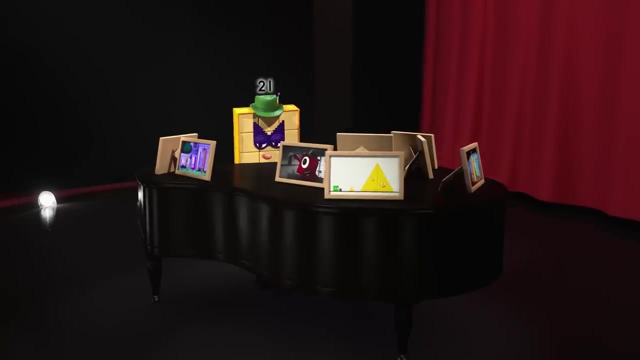 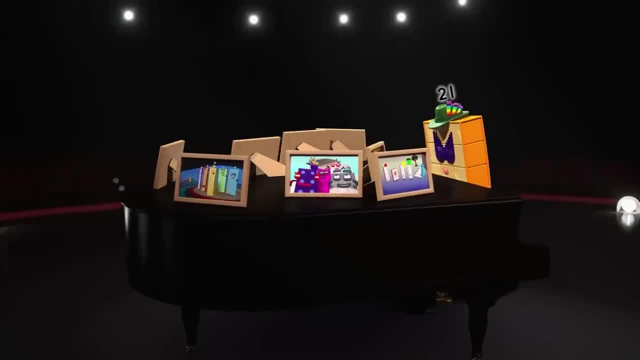 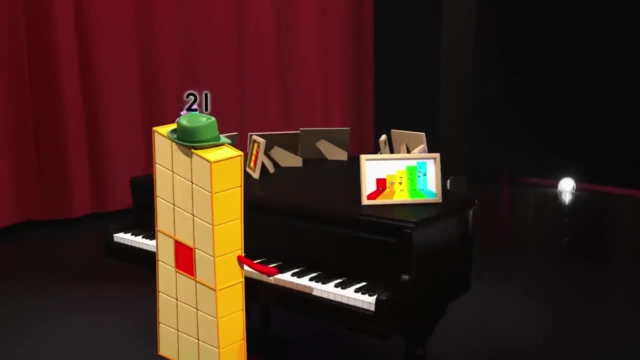 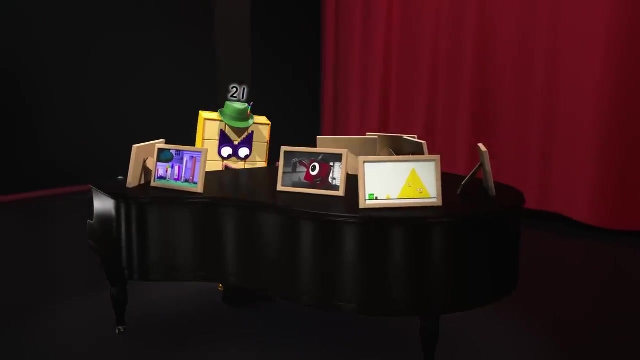 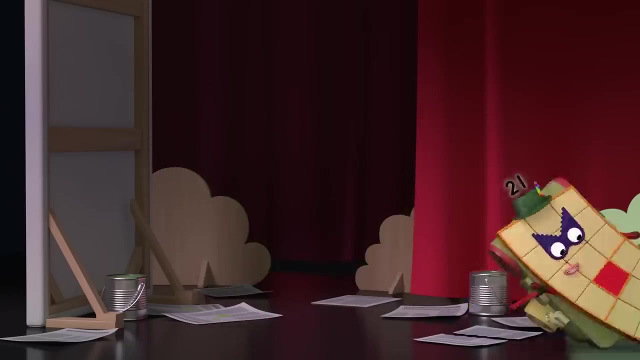 Oh, Oh Oh. We've had such a lot of big adventures And everyone has played their part. Now it's time to take your turn. You'll be happy to learn. This is not the end. It's the start. There's so much more to explore. 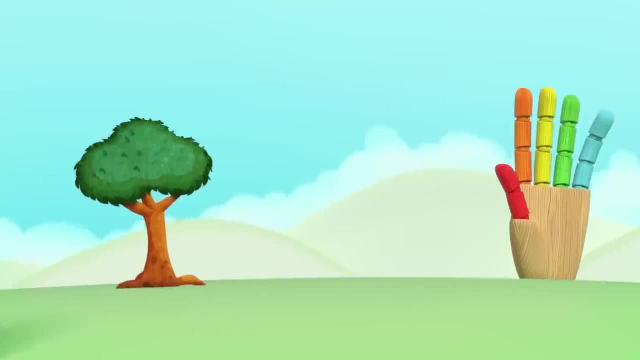 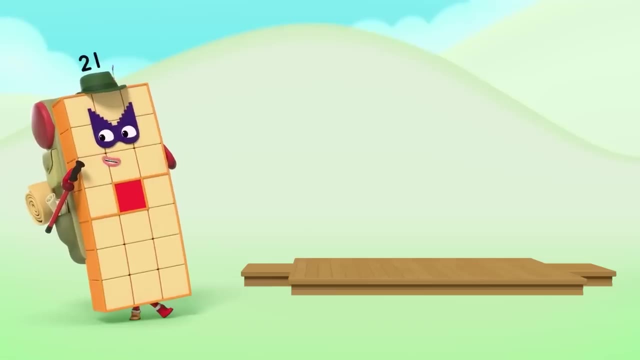 You can take a look Now. we've opened the door. When we ran out of fingers, Unless we counted our toes. how high can we go to? Who knows, If you start with a number for fun, Ha ha, Yeah, You can make it bigger if you just add one. 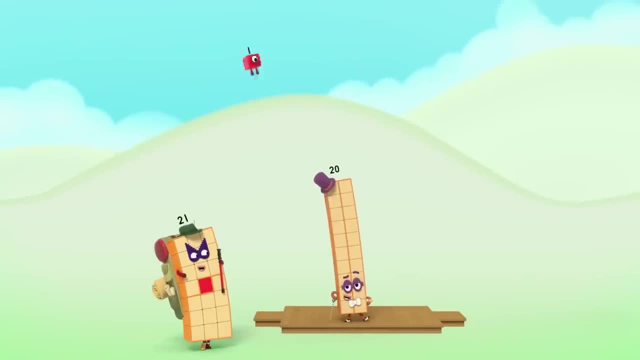 If you just add one, You can do it yourself. Now you know how it's done. Take the floor. There's so much more to explore. There's so much more to explore. You can add a clock, As you've done it before. 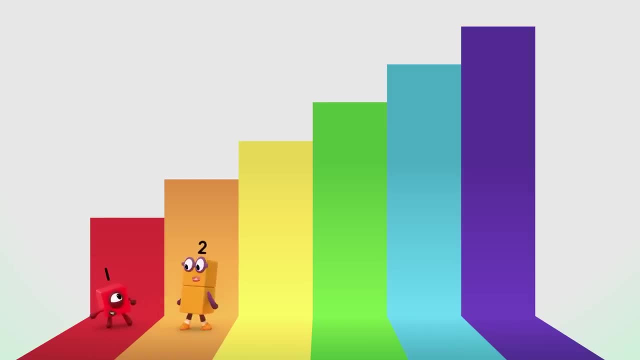 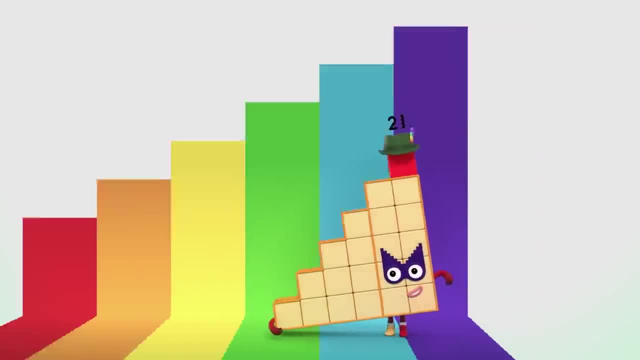 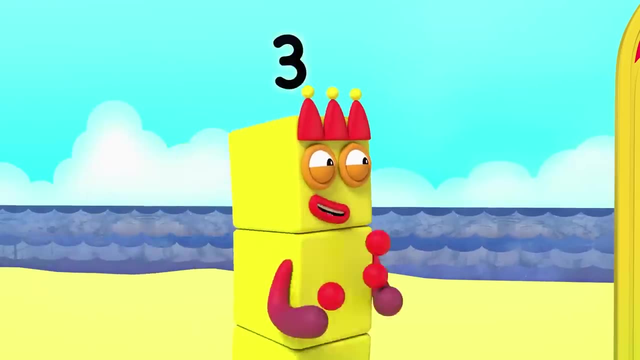 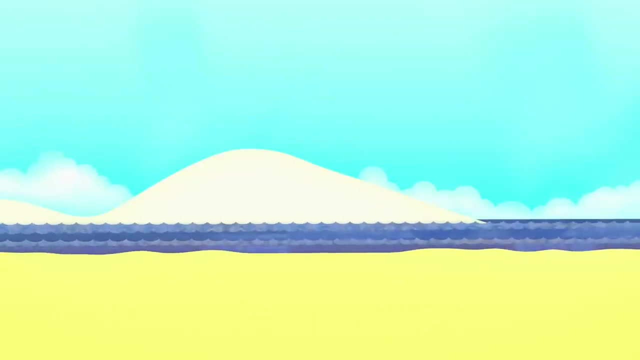 There's going to be magic, No end. It's a plus. you've got us on your side. Soon you'll find your fortunes will be multiplied. You've got all of the tools they took to you to decide whatever. There's so much more to explore. 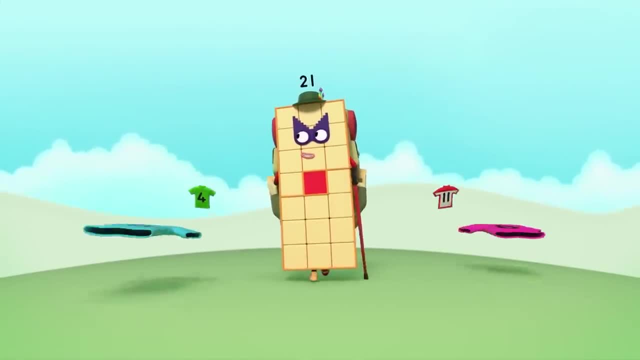 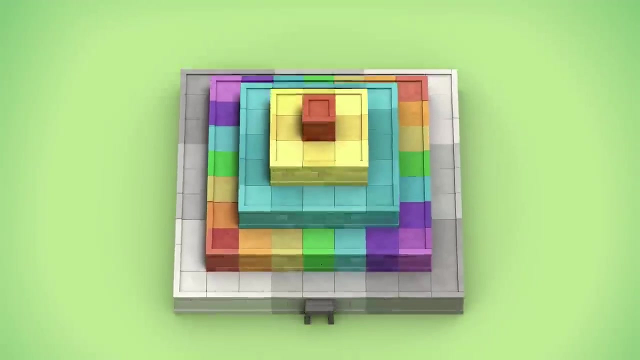 Numbers are everywhere. everywhere you look, You'll find some of us On a clock, On a bus, On the pages of a book. Look at it. There's so much more to explore. Many other squares you've not noticed before. When you know that a square is as wide as it's tall. 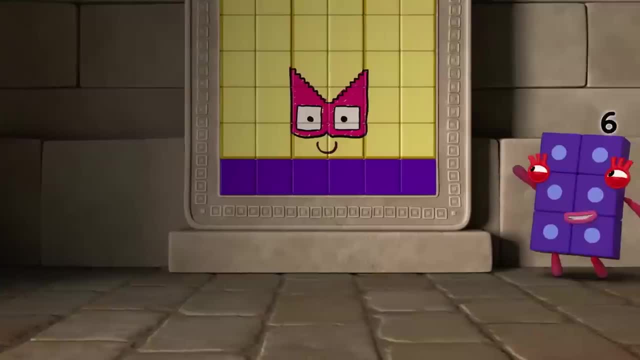 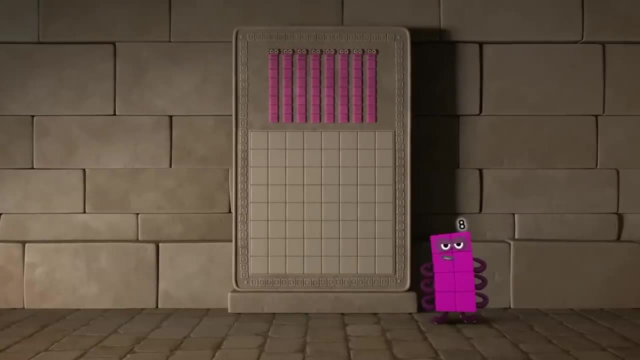 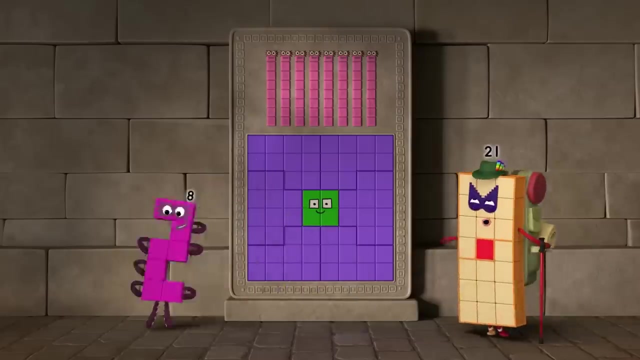 We can make new ones. get tall. Six by six is the next one in line. Thirty-six, Seven tall by seven wide is forty-nine, And I bet you can guess the very next one is mine. Watch me draw- Octoblock draw. There's so much more to explore. 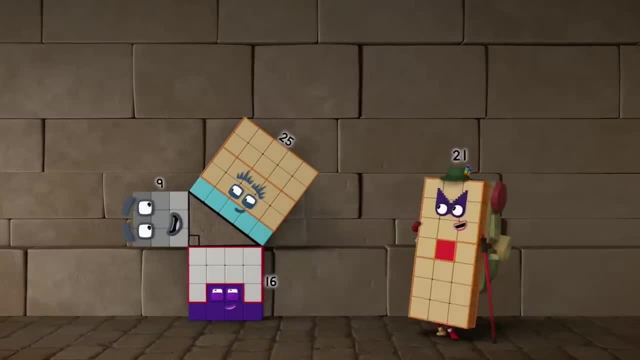 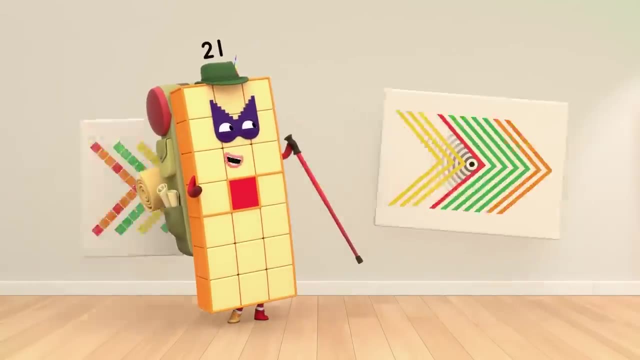 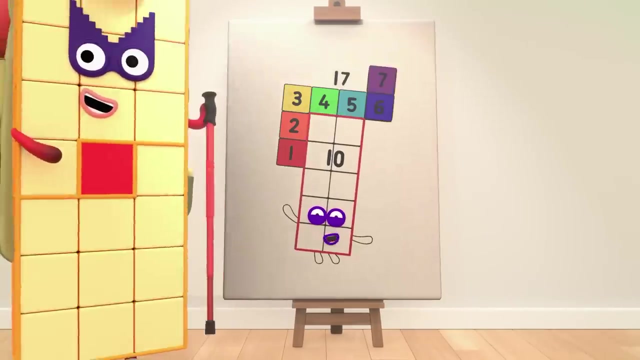 There's so much more to explore: Polka dots, potato prints and patterns galore. So pop on an apron and brush up your art. Painting by numbers- good start. There are so many patterns to spot. Take it step by step and you can learn a lot. 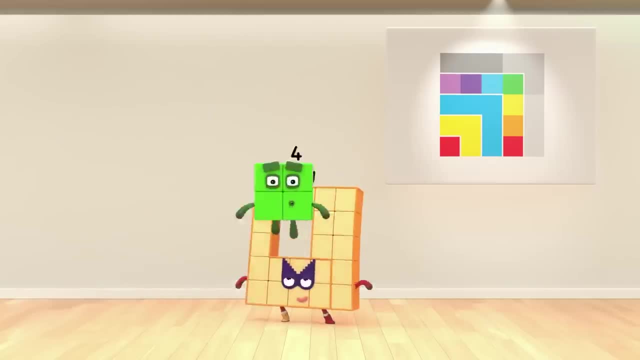 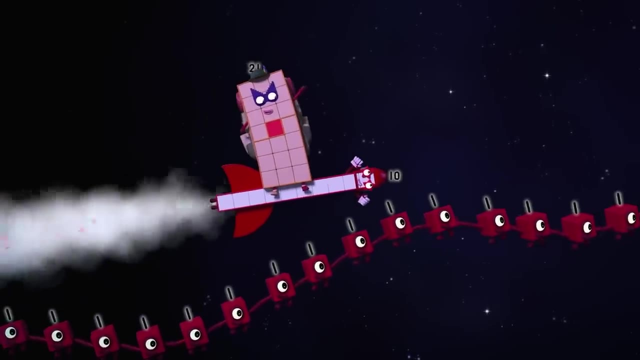 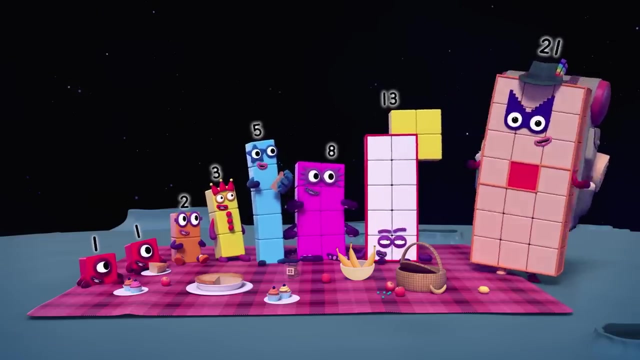 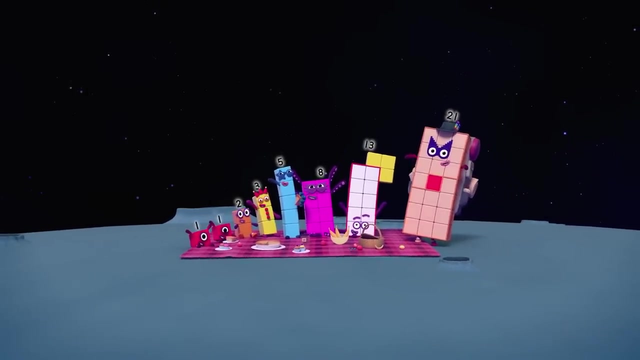 You can shout on your rooftops. now give it a shot. Tell me more. There's so much more to explore. Numbers are infinite. Numbers never end. Keep on and you'll find a mistake in your mind, And we'll always be your friends, Your friends. There's so much more to explore. 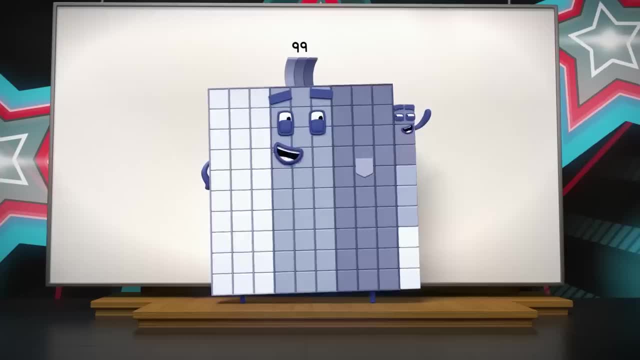 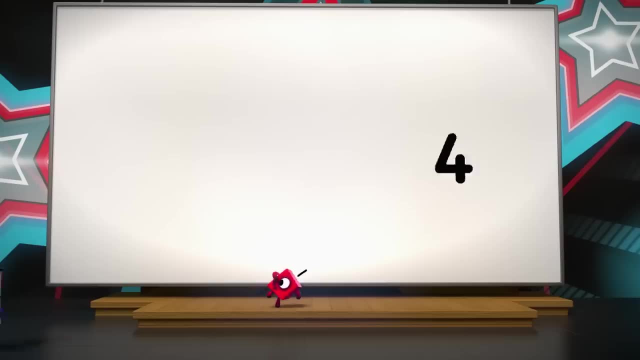 You'll be in the know when you know what's in store. You can count to a hundred By taking it slow. Count to a million. One, two. let's go. Stick with us. put it all to the test. Put two and two together and you'll get the rest. 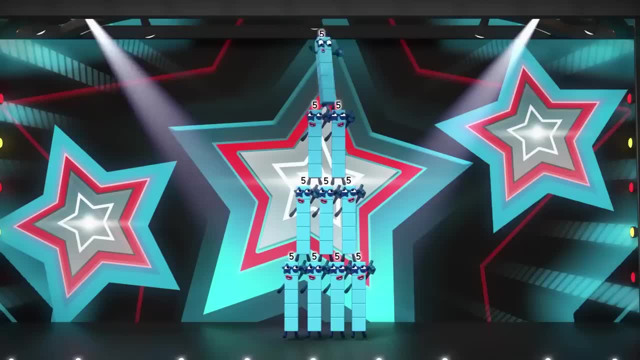 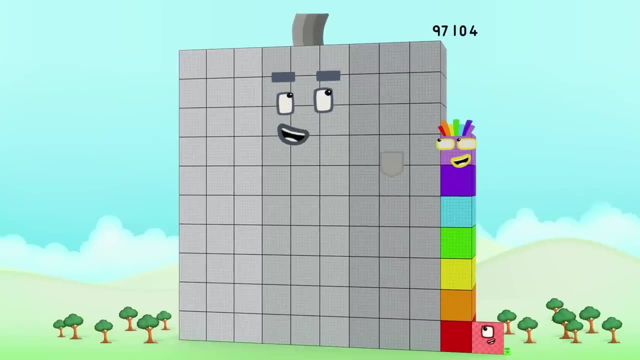 You'll be better at sums than your chums would have guessed. that's for sure. There's so much more to explore. There's so much more to explore Like ninety-seven thousand one hundred and four. Can you think of a number that you've never met? 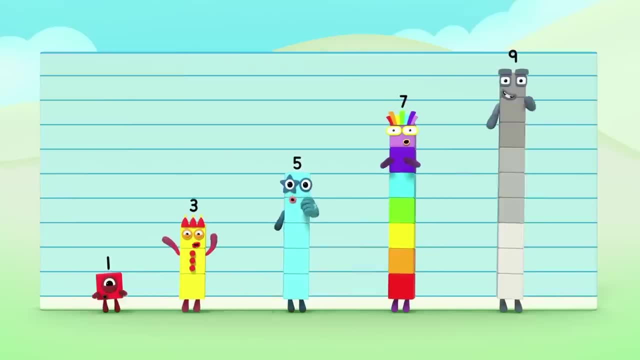 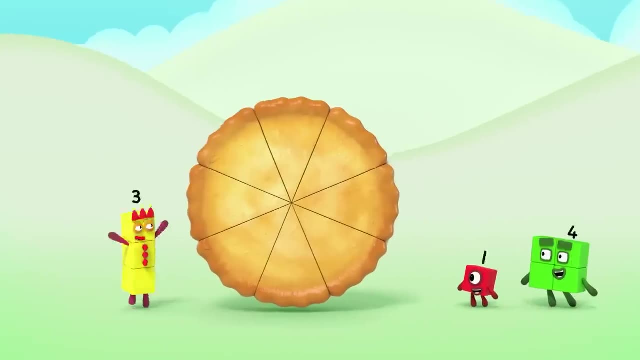 You may go on forever. Two Can you bet? There are all kinds of questions to try. Tell us on a jumper, in a safe, how high And how big of a portion is my piece of the pie? My oh my, don't be shy. 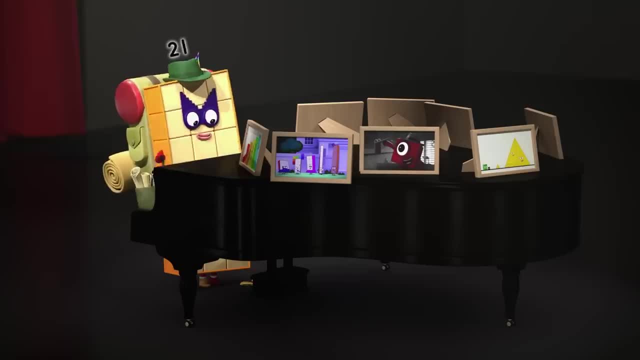 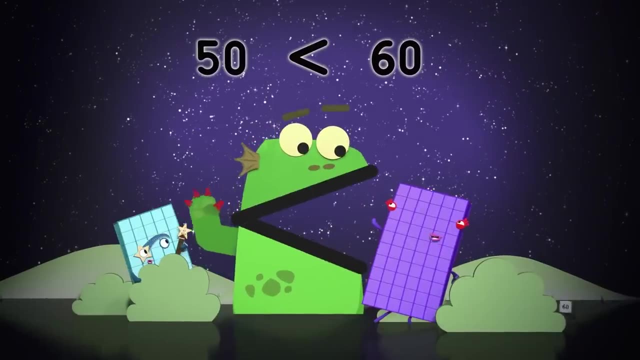 Pick up a pencil and give it a try. We gave you a start so you'd know what to do. You've seen how it works. now it's over to you. So much to discover, so much to seek out Zeros and heroes to learn all about. 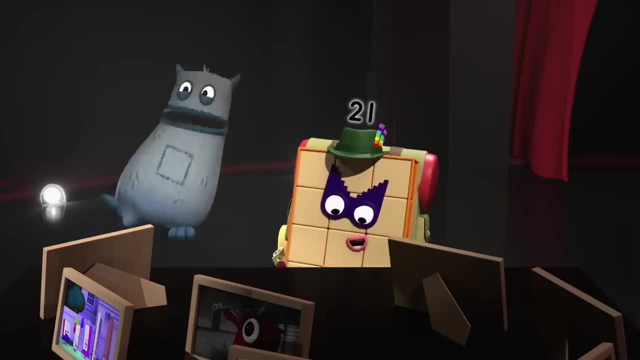 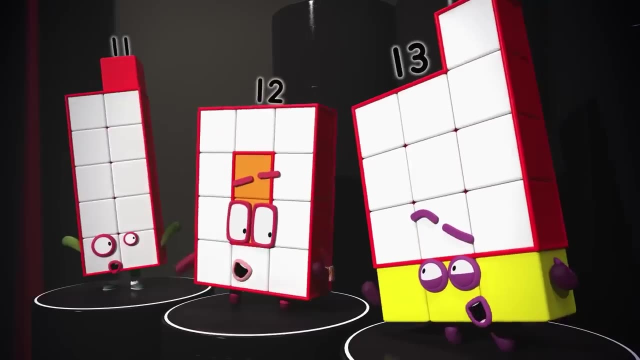 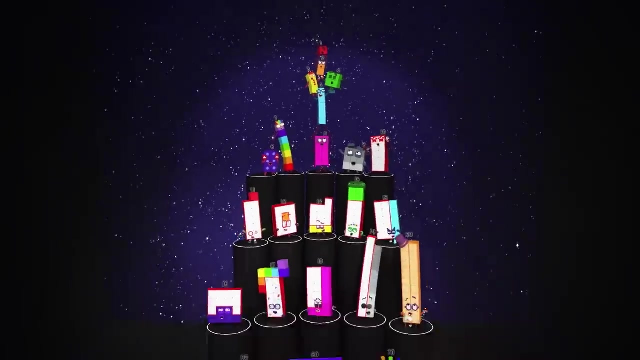 With puzzles and patterns and pictures to pick. You won't miss a moment, you won't miss a trick- Think of a number- and you can be quick on the draw, For there's so much more to explore Your turn.